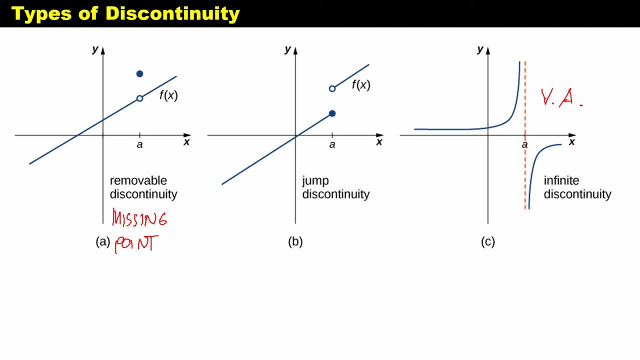 identify the point of discontinuity and its type. Well, that is a very tedious process, So in this lesson, I will be teaching you how to identify the point of discontinuity and its type algebraically. Now, before we move on to our examples, let me share you some pointers on how. 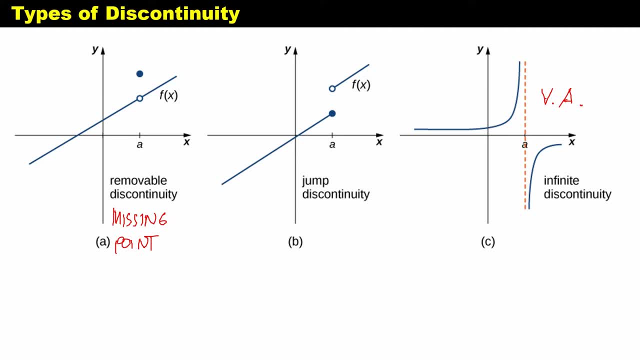 to identify the type of discontinuity Now, if in a given function, for example, you have f of x and then you have x plus 1 in the numerator and then x plus 1 in the denominator and x minus 1. If there is one term or more that you can cancel out, 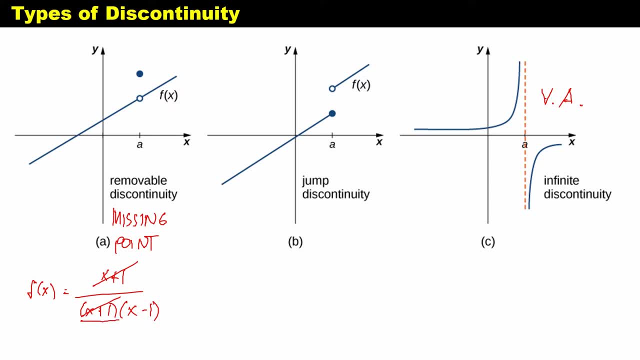 that means that this particular factor, where your point of discontinuity is, is called a missing point discontinuity, since you have cancelled it out using a factor in your numerator. Now, if you say job discontinuity, that happens usually when your function is a piecewise. 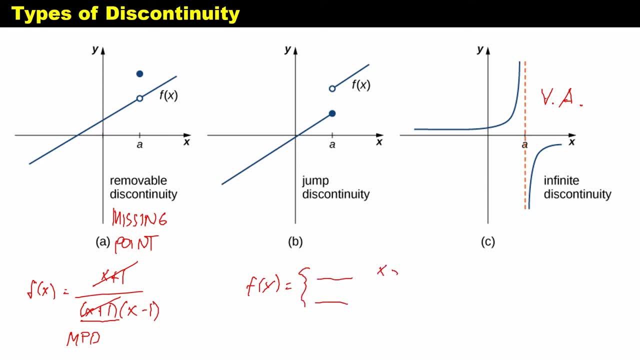 function. say you have something And x is greater than 0, x is less than 0, blah, blah blah. So if you are given a piecewise function, that is a jump discontinuity. Now if you have your function f of x and you are not able to cancel out any term in your numerator or denominator, 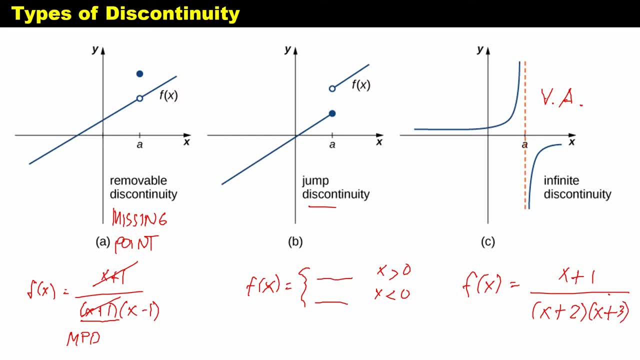 say, we have an example like this: no similar terms. that means that these points of discontinuities are infinite discontinuities And the values of x here, if you equate them to 0, are your vertical asymptotes. So let's move on to our example. 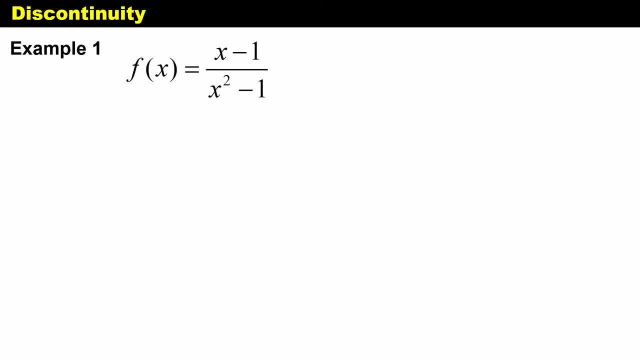 First is: the function f of x equals x minus 1 over x squared minus 1.. Now always remember that discontinuities- discontinuities- happens only if your function is a rational function and if your denominator becomes 0. That means that when we are looking for the points of discontinuities, 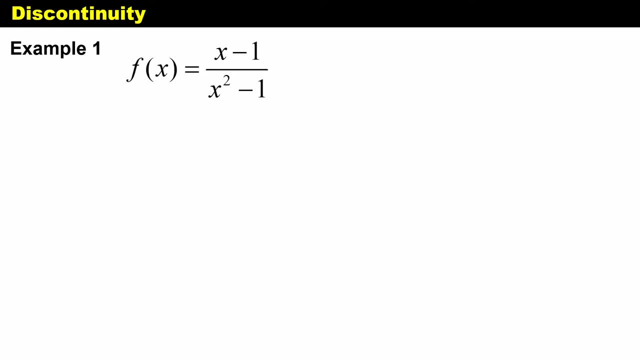 all we need to do is to deal with our denominator and equate that to 0.. So whatever values that can make our denominator be equal to 0 are your points of discontinuity, And then we will be identifying what type of discontinuity are they. 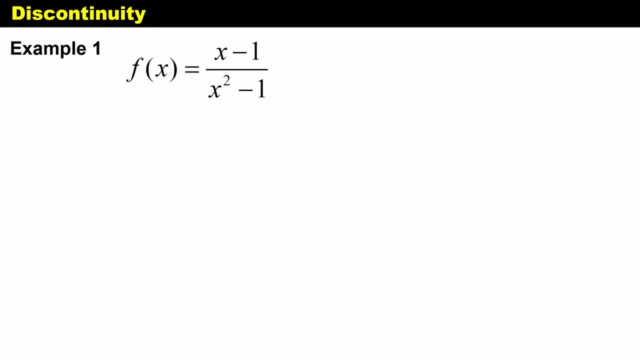 So first we will be looking for the points of discontinuities And then we will be looking for the points of discontinuities. So, for example, number 1, let's try to factor out first our denominator, Since it is factorable, we have x minus 1.. 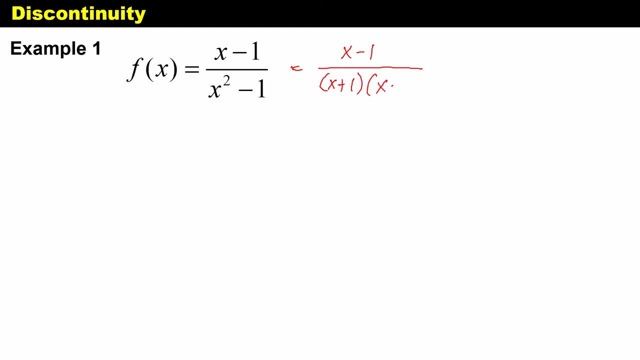 And our denominator's factors are x plus 1 and x minus 1.. Now, as I have said earlier, we have to equate our denominator to 0. So this becomes: x plus 1 equals 0 and x minus 1 equals 0.. 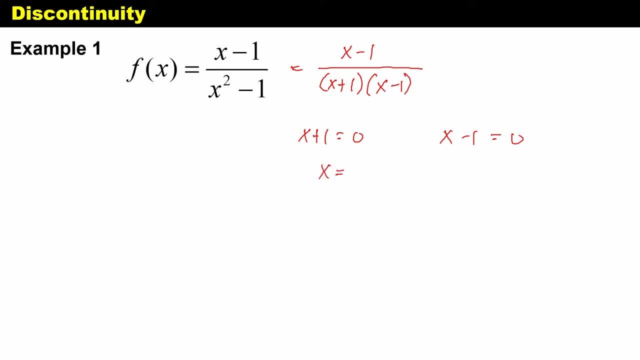 Now, if we equate our denominator to 0,, we have to equate our denominator to 0. So if we isolate positive 1, this becomes negative 1.. And then this becomes positive 1.. So these two points are our points of discontinuities. 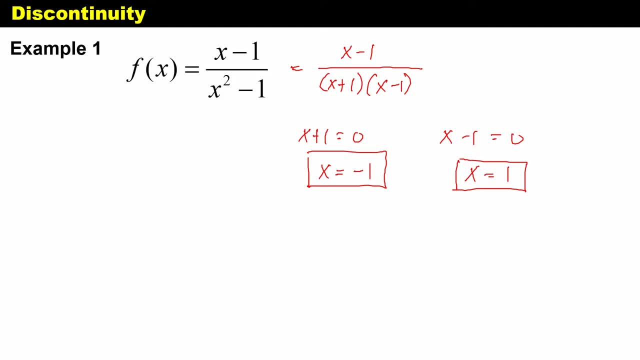 Now we will be identifying the type of discontinuities of each of these points of discontinuities. Now let's go back to our function And, as we can see, we can actually cancel out x minus 1.. That means that x equals 1 is actually a missing point. 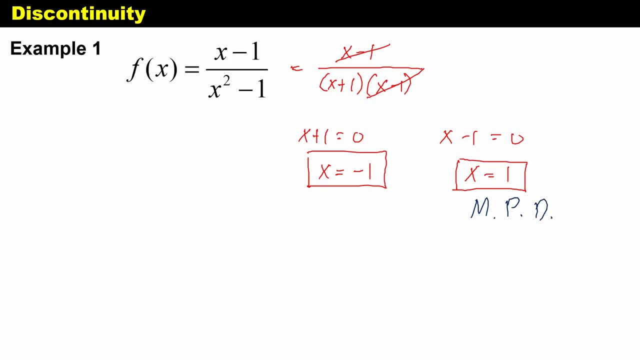 Now we were not able to cancel out x plus 1.. That means x equals negative, 1 is an infinite discontinuity. So that is how you solve for the points of discontinuities and identify its type. Now let's move on to our second example. 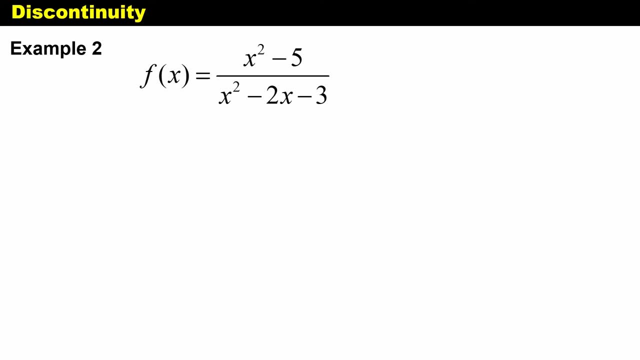 Now we have f of x equals x squared minus 5, all over x squared minus 2x minus 3.. Now, as what I have said earlier, if we can still factor out our numerator and denominator, then we have to factor out. 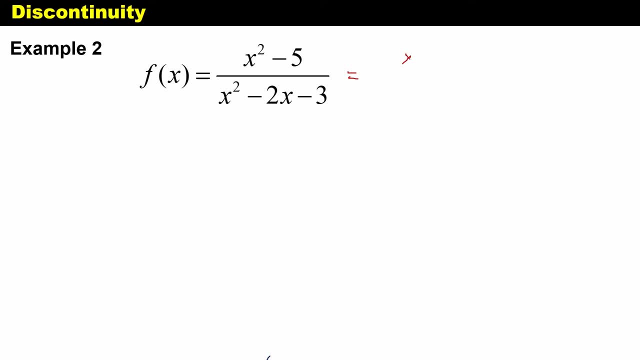 So since our numerator cannot be factored out anymore, we will just copy x minus 5.. Now our denominator's factors are x minus 3 and x plus 1.. Now next step is to equate Our denominator to 0.. 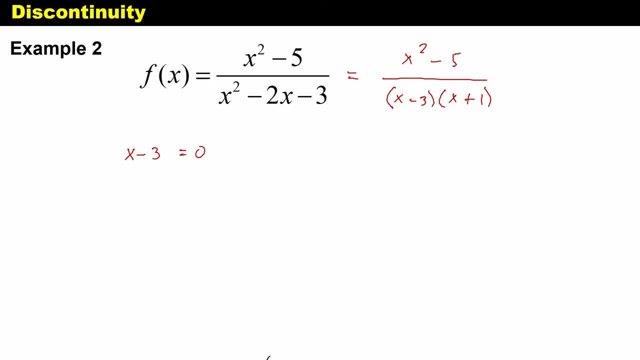 So we have x minus 3 equals 0. So we have x equals positive 3. And x plus 1 equals 0. So we have x equals negative 1.. So we have these points of discontinuities. Now let's try to identify its type. 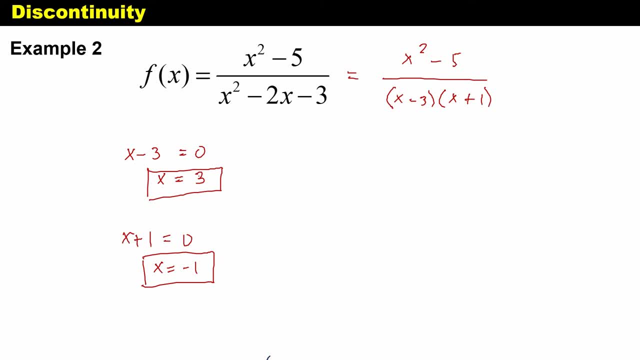 Now, since we were not able to cancel out any of them in our function, that means it's Its type is an infinite discontinuity. Another example: we have f of x equals x plus 1, all over x squared plus 2x plus 3.. 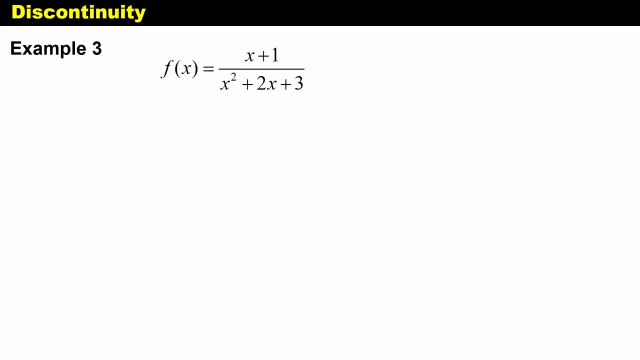 Now observe that our denominator x squared plus 2x plus 3, cannot be factored out. So what we're going to do is to check whether our denominator has real roots or imaginary roots. Now, how do we identify if our denominator has real roots or imaginary roots? 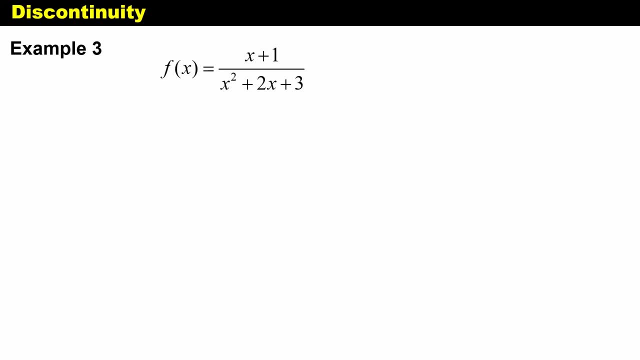 We will be using the determinant formula b squared minus 4ac. Now, if the value of your denominator becomes greater than 0, that means you have two real roots. If that is equal to 0, that means you have one real root. 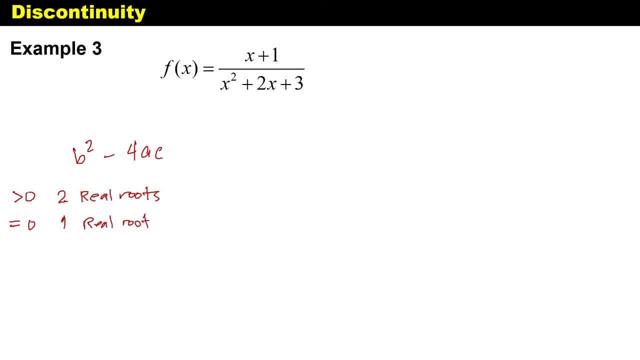 And if the value of your denominator becomes less than 0, that means you have two imaginary roots. Now let's try to use this formula and identify whether our denominator has real roots or imaginary roots. So our a becomes 0.. So our a becomes 0. 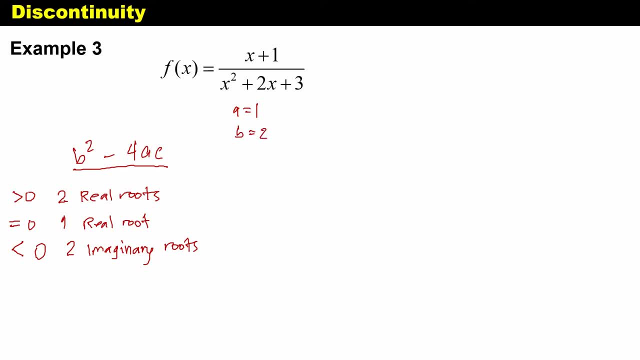 So our b becomes 1.. b is 2. And c equals 3.. These are just the coefficients of x squared 2x and the constant 3.. So this becomes 2 squared minus 4 times 1 times 3.. 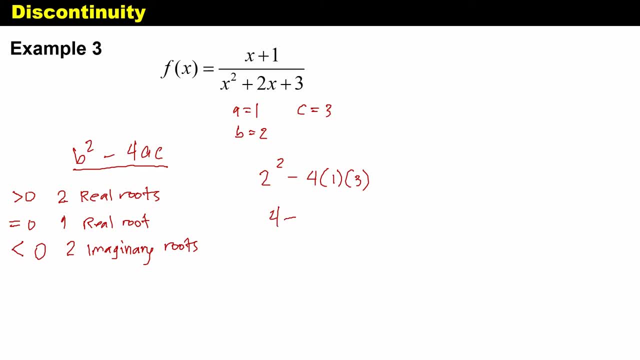 We have 4 minus 4 times 1 times 3 is 12. So the answer is equal to negative. So the answer is equal to negative 8.. Now negative 8 is less than 0. That means we have an imaginary root. 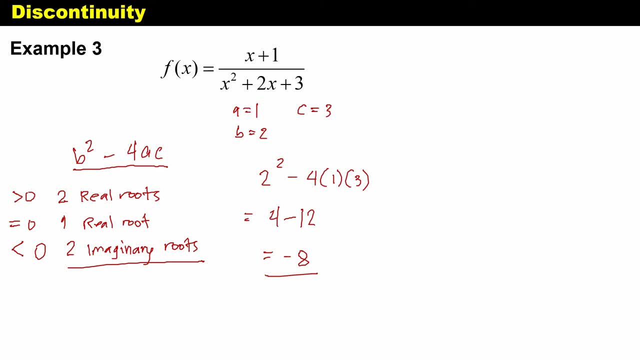 Meaning there is no particular value of x that can make our denominator equal to 0. This means that this function is actually continuous, So there are no points of discontinuity. Again, if you cannot make your denominator equal to 0,. 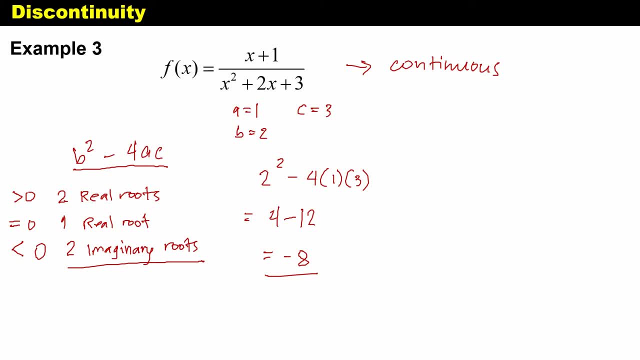 that means your function is continuous And there is no point of discontinuity. Now let's move on to another example. We have the f of x equals 3x squared minus 3, all over x cubed minus 5x squared plus 2x plus 8.. 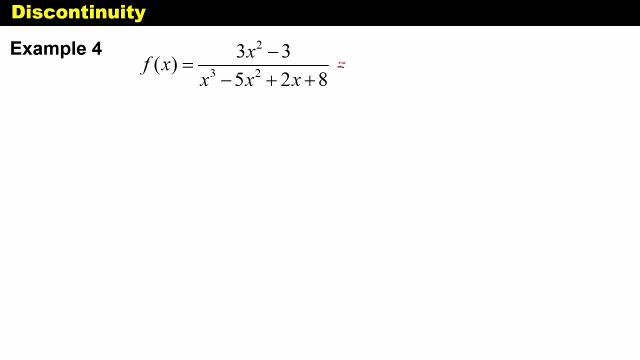 Now what we're going to do is to factor out our numerator and our denominator, So we can actually extract 3.. So we have x squared minus 1.. And we know that x squared minus 1 is difference of 2x. 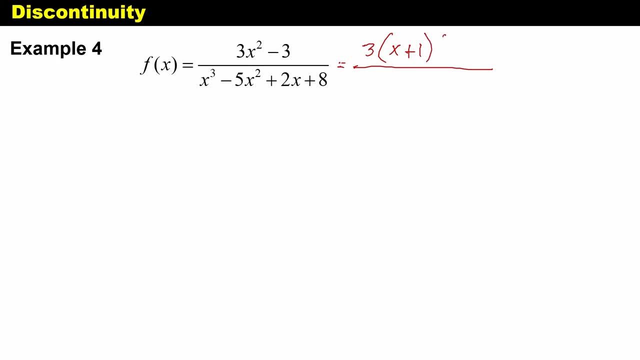 So we can factor out x plus 1 and x minus 1.. So these are the factors of our numerator. Now let's move to our denominator. Our denominator is quite hard to factor out, So let's use synthetic division. 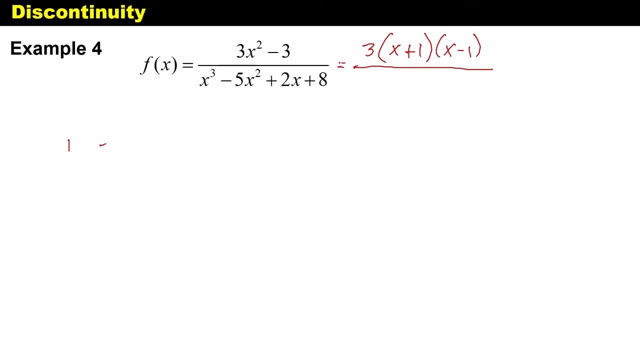 Let's copy their numerical coefficients. We have 1, negative, 5, positive, 2, and positive, 8.. And then Let's look at the factors of our last term, or the constant term. We have 8, 1, negative, 8, negative, 1,, 4,, 2, negative, 4, negative 2.. 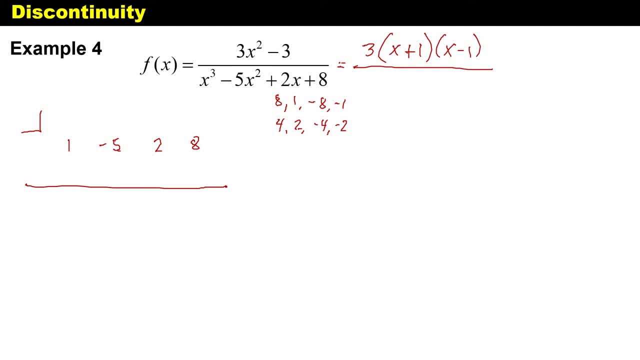 So let's make use negative, Let's try negative 1. So negative, 1. This becomes 1.. 1 times negative: 1 is negative 1. Negative 5 plus negative: 1 is negative 6. So this becomes positive 6.. 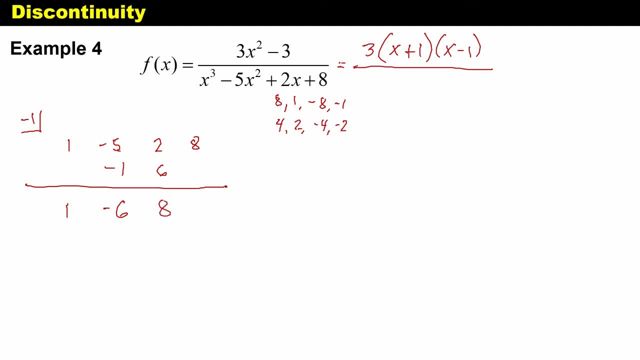 And then positive 8.. 8 times negative 1 is negative 8. And this becomes 0. So this cancels out. So 1 root is negative 1.. Another is: This becomes x squared minus 6.. 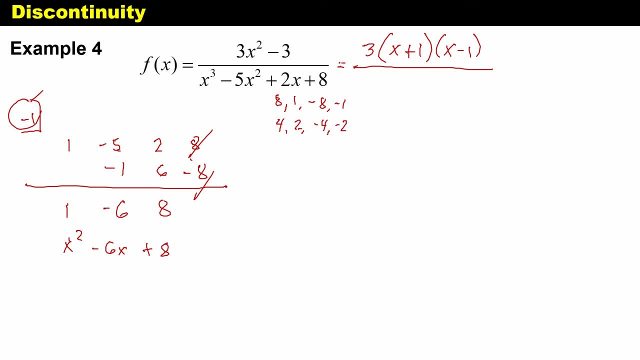 This is x plus 8. Now we can already factor this out. We have x minus 4 and x minus 2.. So if we equate this one to 0.. So this one is already. x equals negative 1.. 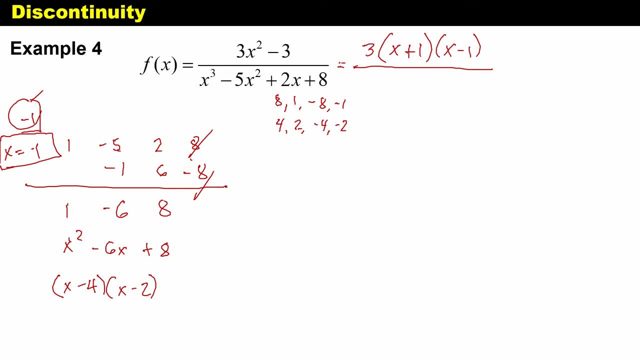 This is already 1 root. Now, if we equate this one to 0,, this becomes x equals positive 4.. And this becomes x equals positive 2.. So we already have our three points of discontinuities. So again, this is x plus 1, x minus 4, and x minus 2.. 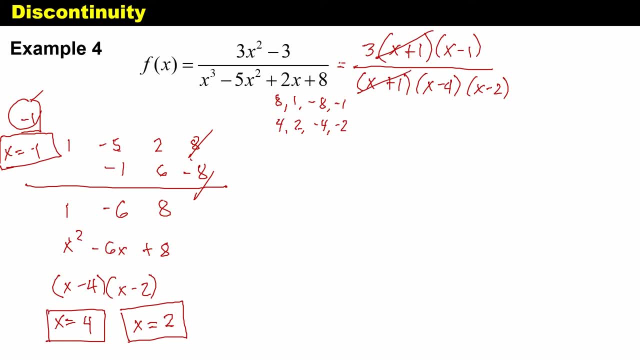 Now we can cancel out x plus 1. here, Meaning this one x equals negative 1, is a missing point. So this is an infinite discontinuity, And since we were not able to cancel out x minus 4 and x minus 2,, 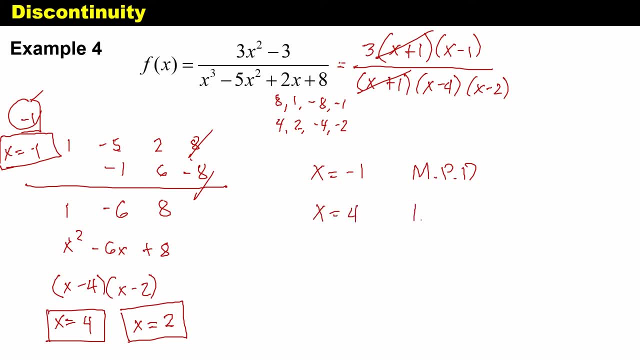 that means x equals 4 is an infinite discontinuity, And x equals 2 is also an infinite discontinuity. So these are our answers. Now let's have this, This example, and as we can see, it is a piecewise function. 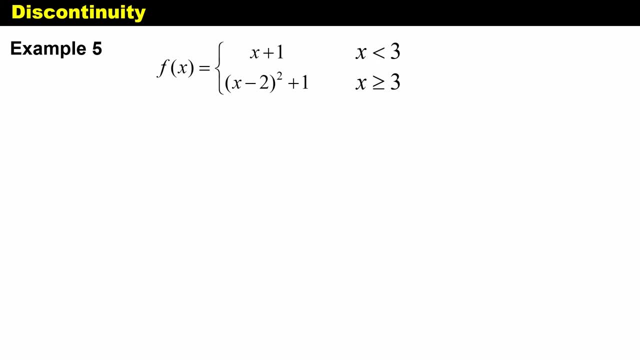 So we already know that this function has a jump- discontinuity- But how do we identify what is the point of discontinuity? So, to identify the point of discontinuity, what you need to consider is the value, or the values that you can see in the conditions given. 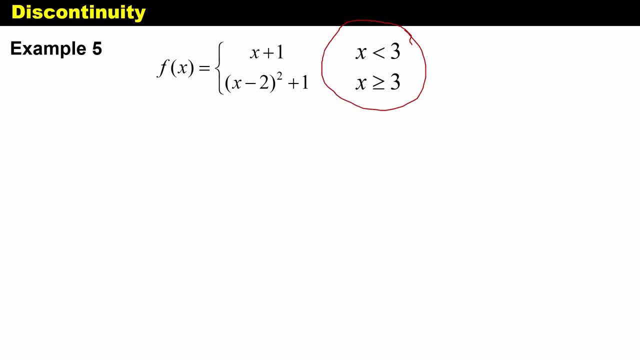 Now, since we only have here 3,, that means our point of discontinuity is at 3.. But if your conditions are, for example, x greater than 2,, and then x is greater than or equal to negative 5, but less than or equal to 2,.